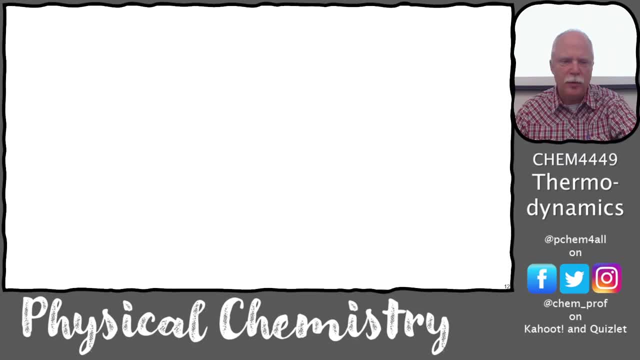 So let me go ahead and snip those, put them into our PowerPoint. Okay, so here's 26 and 27.. So that's going to be on the viscosity chapter. So let's go up here and look, And I would go to my note card. 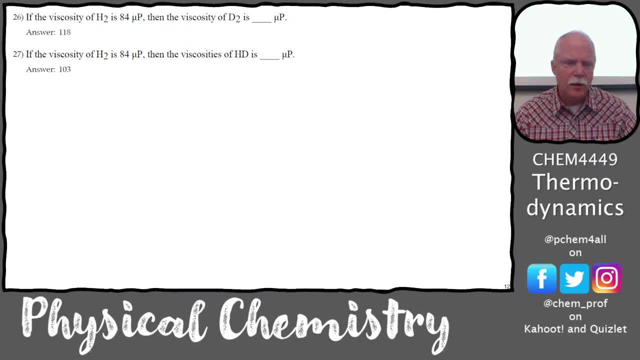 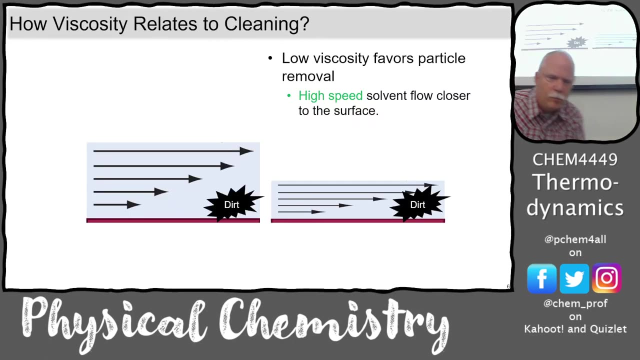 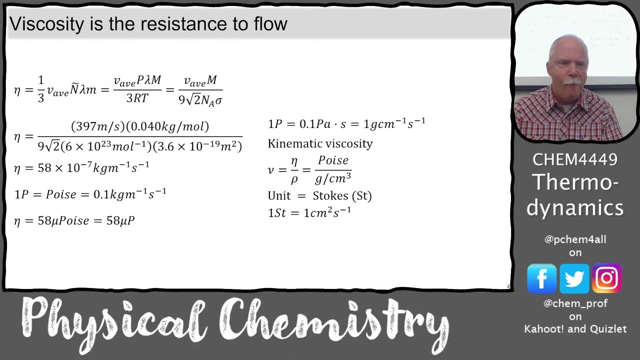 Let's see. if you guys don't have that shown, Let's do this, Let's work our way backwards, And so here's a: looks like a direct dependence on mass, but also mass is in the velocity. Okay, so we've got a couple of mass dependencies. 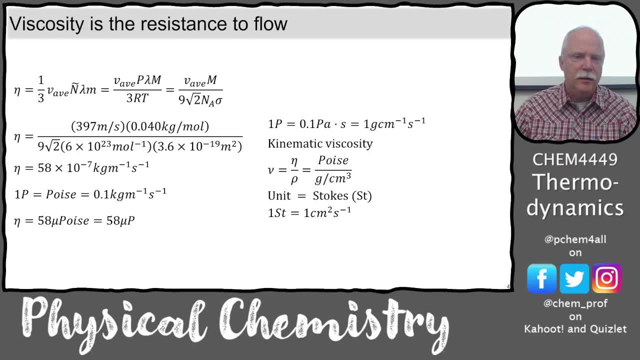 And so let's break that into the pieces. Okay, so we've got. Okay, so we've got, Let's just do it right here. So we've got mass dependency here. I'm going to have to figure out how to mark off the area on my little pad here. 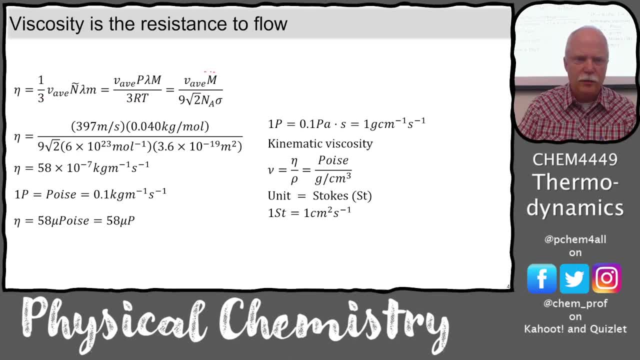 so I can find my pen Here. it is All right. so let's look at this right here. So viscosity is proportional to these two items here, and the mass is in both of them. Okay, Okay, and so The average velocity. 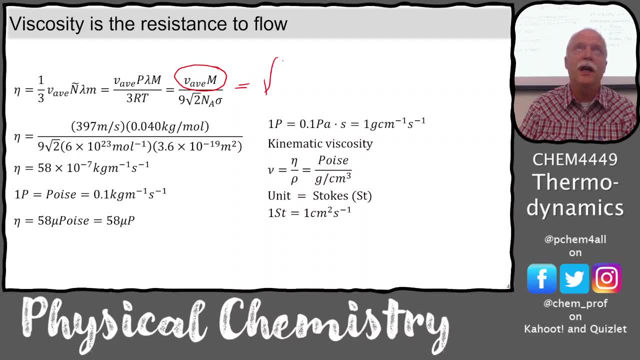 Let's see: most probable is 2.. The average was 8 over pi. Remember that? Yeah, so it was 8 over pi, RT over m. So that's the average velocity. It was most probable was 2 RT over m. 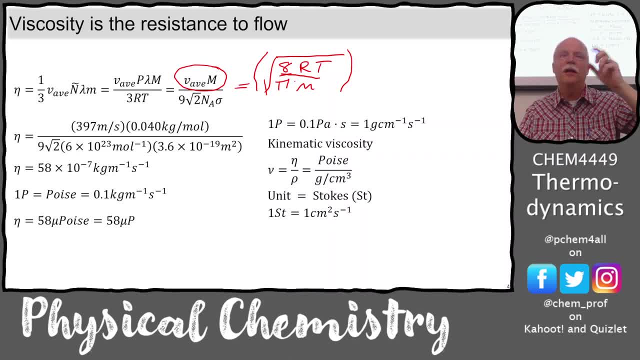 and the- I mean squared was 3 RT over m and this is the one in between. Okay, and then we have m here over this business, 9 to NA sigma. So what we're trying to figure out is: how is viscosity proportional to mass? 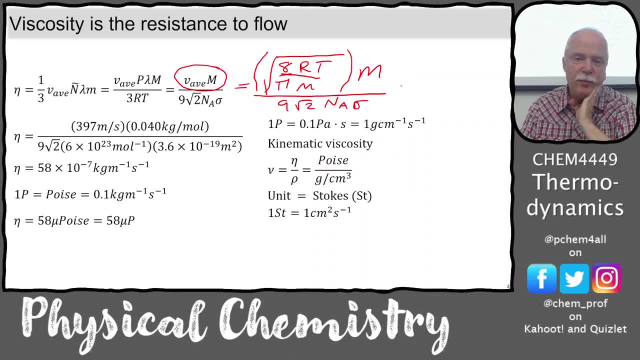 Okay. So just looking at this, we would say it's proportional to mass over the square root of mass. Does everybody agree with that? I've got a square root of mass here in the denominator and then I've got a mass in the numerator. 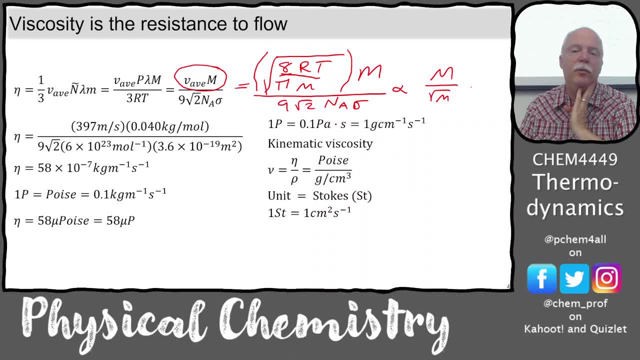 Okay, So it would be proportional. then How would that cancel? Well, this one is the square root of mass, squared right on top, and so it's proportional to the square root of mass. It's not very well written, but you understand what I'm saying. 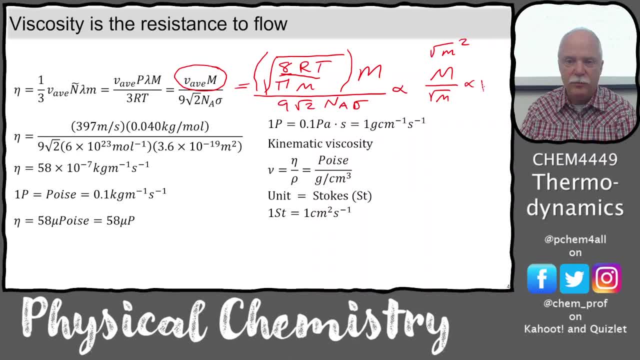 so let me clean it up a little bit. So viscosity is proportional to the square root of mass, And so we can do: eta 1 over eta 2 is equal to the square root of mass 1 over the square root of mass 2.. 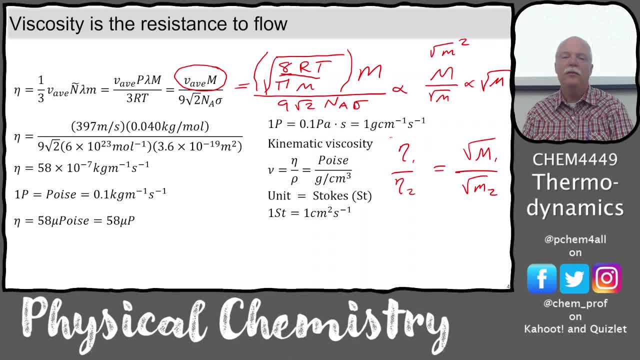 So you see how, even though we don't know the cross-sectional area, we don't know, I mean, we could figure out all the other constants- pi and r and everything. We don't know what the temperature is, but this is all we need to know. 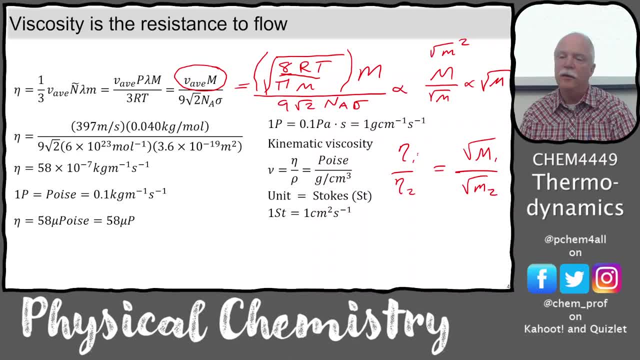 We're saying, at the same temperature, what's the new viscosity? Okay, So let's solve this I like to do. you know, situation 2 is the new molecule, so situation 1, so it would be eta 1.. 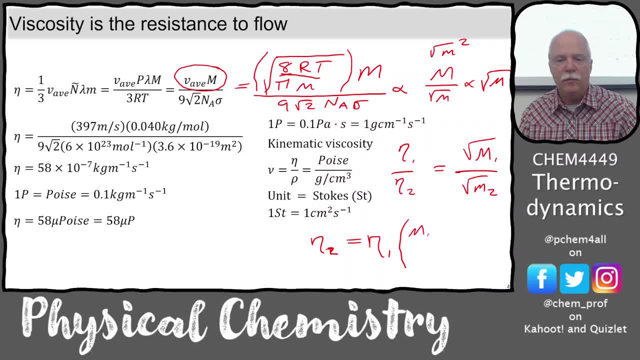 And so then that's going to be m2 on top and m1 on bottom, All to the one half. So then we could go to our problem and put those numbers in. So what was the viscosity for h2? 84.. 84.. 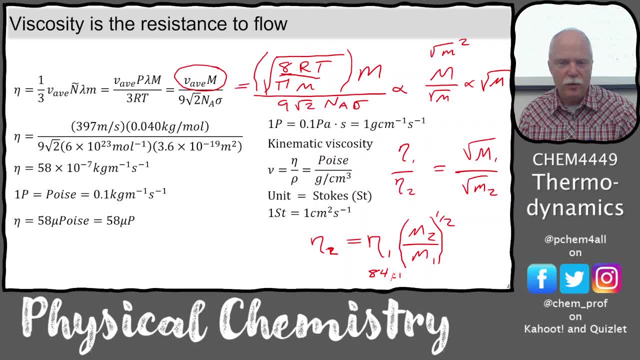 Centipoise, Or what was it? Micropoise, Micropoise, And then it was d2.. So we could use 2 for that. So 2 on top No 4, right 4.. D2 and 2 for hydrogen. 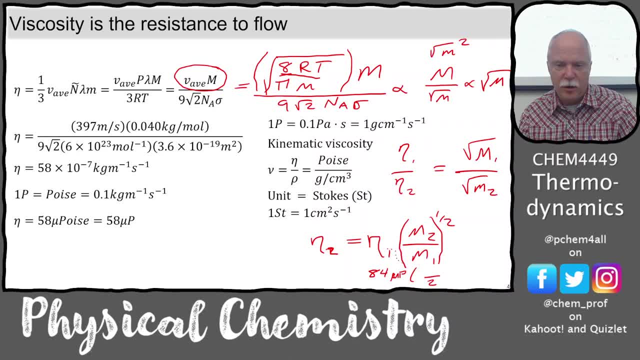 Those are our masses, All right. So the square root of 2 is 1.41 times 84.. So hopefully it's 118, because that's what the answer is. Okay, Yeah, the same kind of problem with the ones and twos, but a little bit of added twist, right, You had. 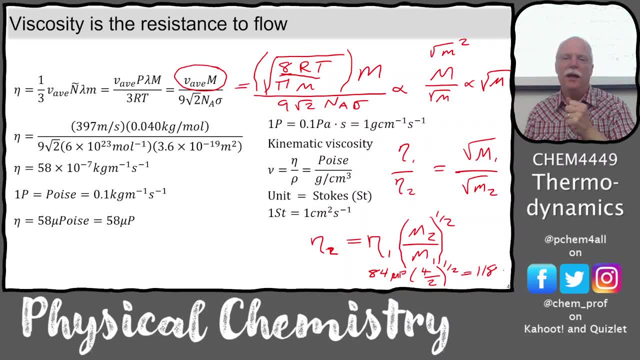 to dig a little deeper to figure out where the mass is and to just see that average velocity, and go, wait a minute. I think there's a mass buried in there somewhere, So you might have to do a little extra work in that case. I think the next one is similar. Okay, great. 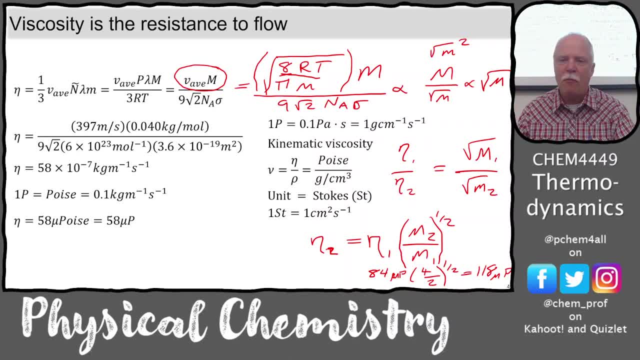 Wasn't that fun. Clock is broken too, isn't it? The one in 123 was broken. Now it's fixed. Okay, what's next? I can't tell. are y'all cautiously optimistic or panicked, or what? Don't want to jinx yourself. 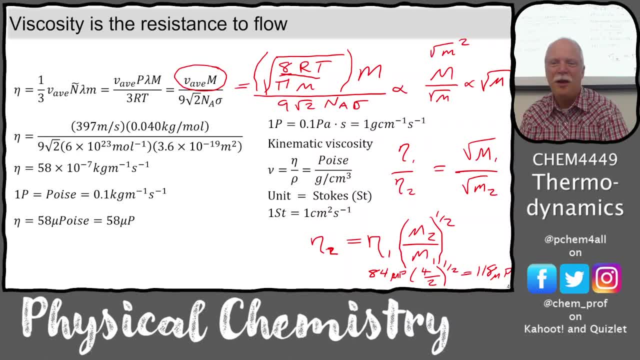 I can't quite pin it, but I'm not Okay, Yeah, I think I got it. what 22?? 22. Okay, I wish I could mark on PowerPoints, but I mean on PDFs, but I can't. 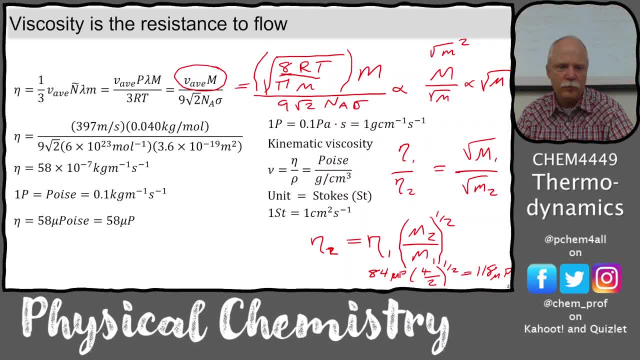 So that's on the fusion. So we'll see, We go, Let's see, let's go, pull those notes out. thermal conductivity and diffusion. that's that set of notes. okay, i've got two powerpoint slideshows going. okay, let's see, let me escape out of that one. 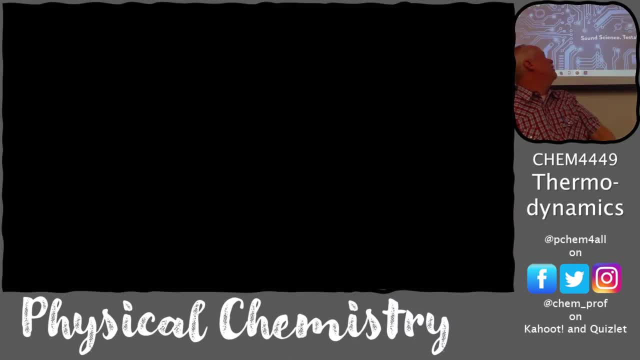 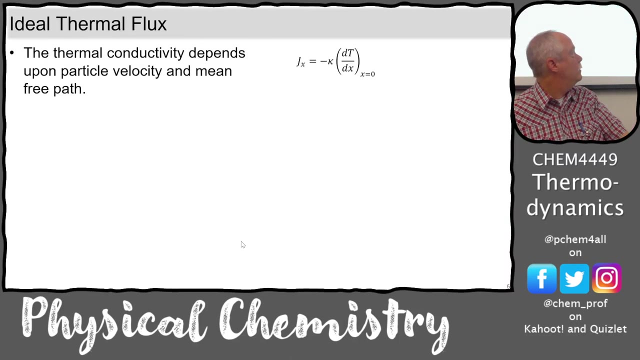 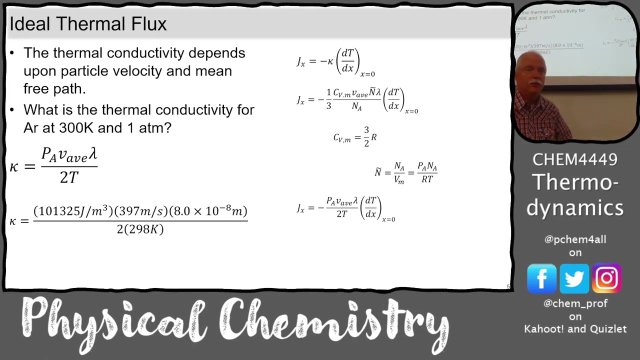 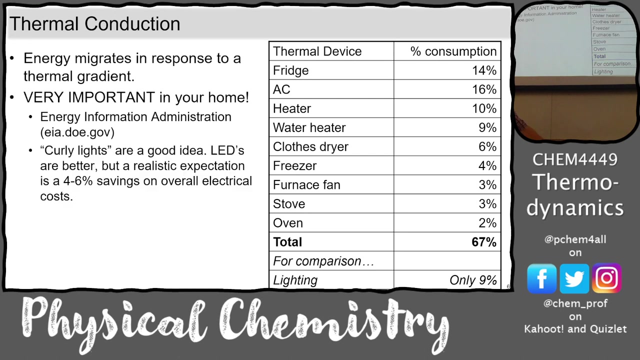 okay, okay, so we're looking for um the diffusion equation. it doesn't look like it's restricted to one one dimension. okay, we're looking for the three-dimensional and we want time dependence. okay, so these are all thermal connectivities. we've got to find the diffusion spot. 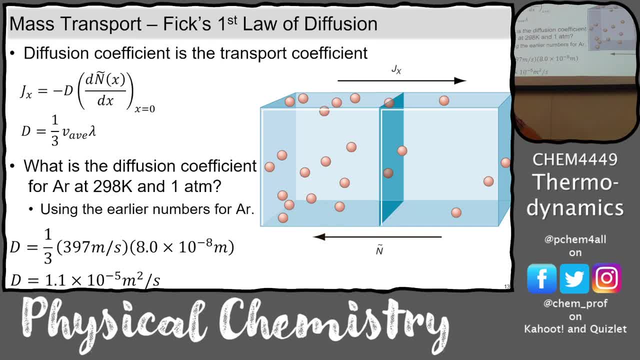 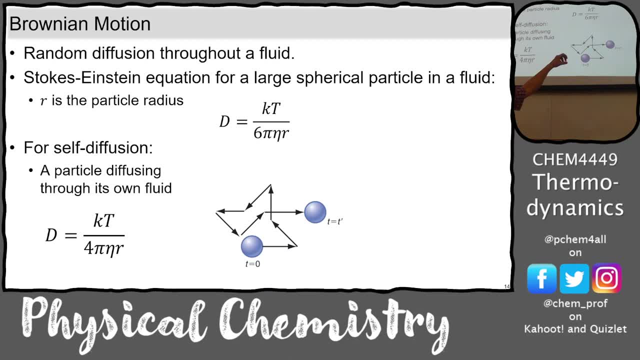 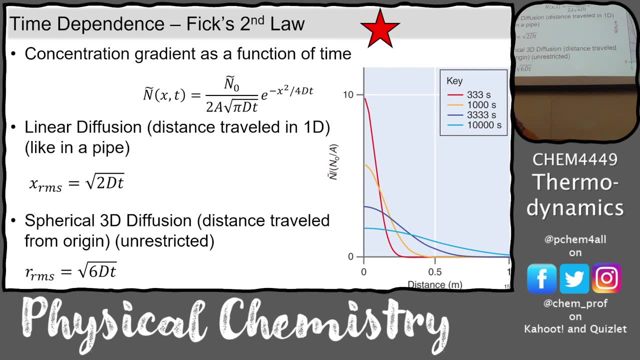 all right, here we are in diffusion. okay, we see velocity there, um. here's related to diffusion, um and based on the particle radius and the temperature. but i don't see any time in there, so we skip that equation. and then here's again the concentration gradient, so it looks like this is the. 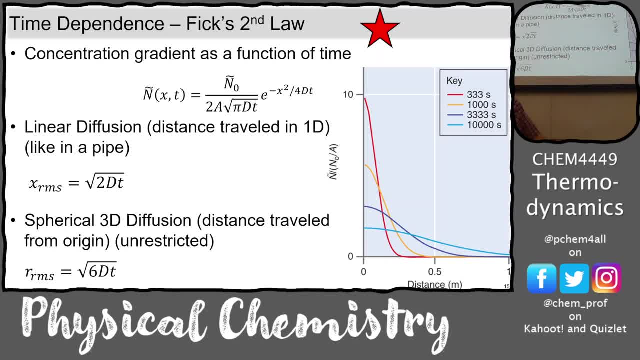 kind of thing we need, and it's the square root of the time. okay, so that's the key right there. we needed to see how far it diffuses, based on the r or x, but both of these are the square root of time. so so we can, we can take that, i can paste. 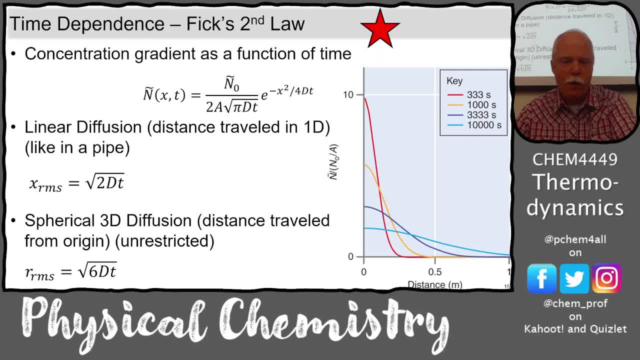 that little question right here. yeah, it worked, can you see it? yeah, okay, great, and so then it's the same kind of key of time. so that's a little bit of time, god, that's the key right there. yeah, that worked, can you see it? yeah, okay, great, and so then it's the same kind of key. 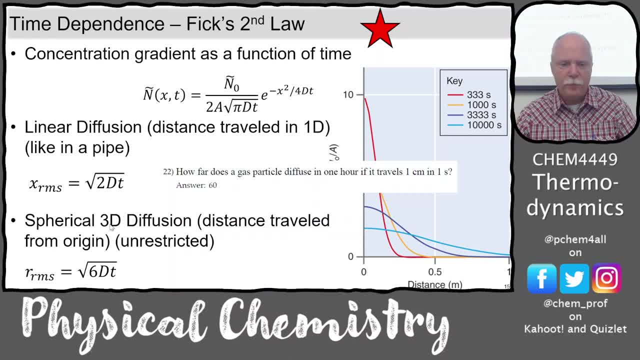 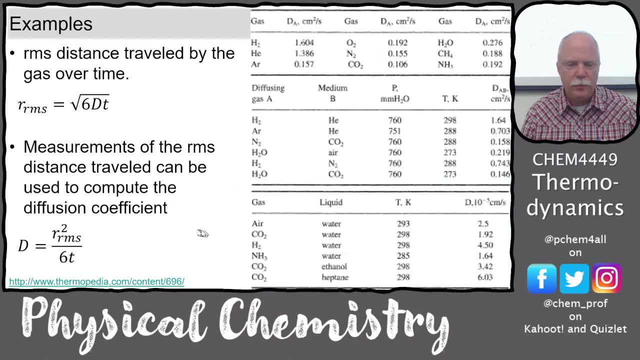 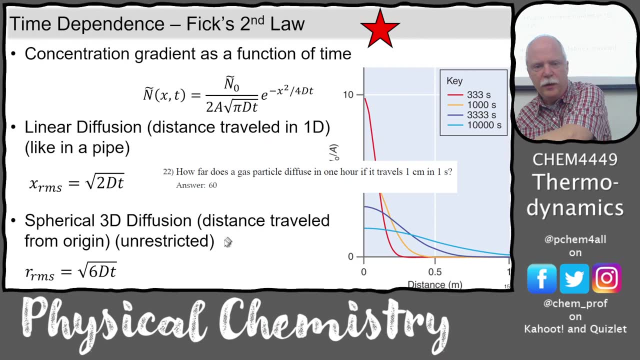 question where it's a square root dependence on time. all right, here we go. where's my pen? what I mean? I see the little arrow, but it won't. it won't mark anymore. yeah there, it is strange. okay, so this is um. R is proportional to time to. 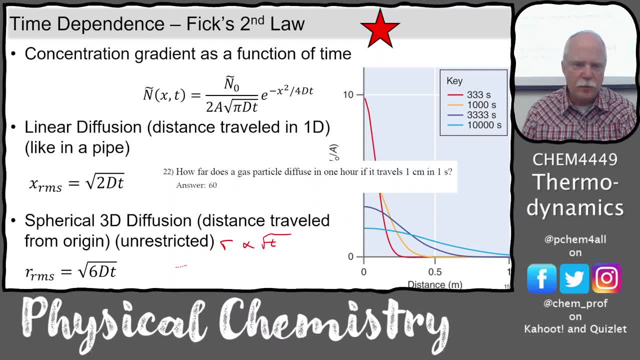 the 1 half power, and so that's one centimeter, okay. and so then we have one hour, so we had one second. one centimeter, one second, okay. and so how many seconds is in in an hour? yeah, 3,600, 60 times 60. if it's 60 times 60, then the square root of that is: 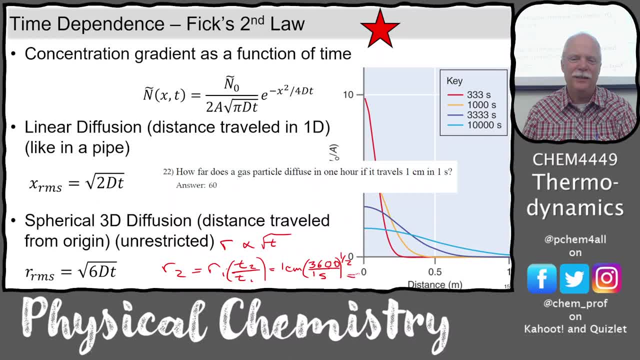 just 60, okay, so that's gonna end up being 60 centimeters. so once you find this- I guess this is again the take-home lesson and all of these equations- is, once you find a proportionality, then doing case one, case two always works, yeah, and you can not worry about what the diffusion constant is or the. 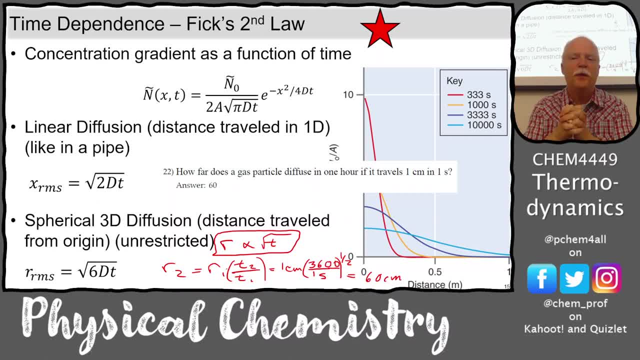 coefficient of six or two or three or whatever you want to call it. and then you can't do anything like that because if those things haven't changed, you're just looking at the proportionality. how to? if I change the thing that is proportional to, and I take into account the proportionality like one half power. 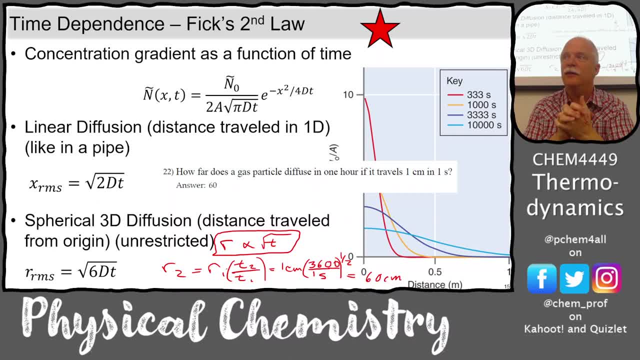 or remember the partition function. that was my favorite one. it was the like the five thirds or something ridiculous like that, or three-fifths power. those were crazy. you know it's Passell's law with the radius to the fourth power. you know that one is pretty interesting. 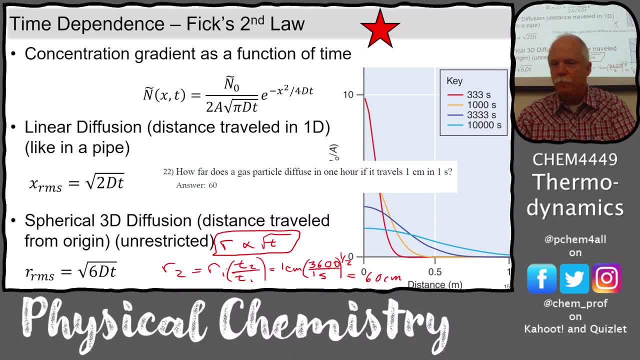 okay. okay, You're talking about how many of these things were 그리고 6. okay, yeah, that means seven. seven is the tough one. that's crazy. so let's see, let me snip both of those, and I always have to. I struggle with seven because it's always a year. 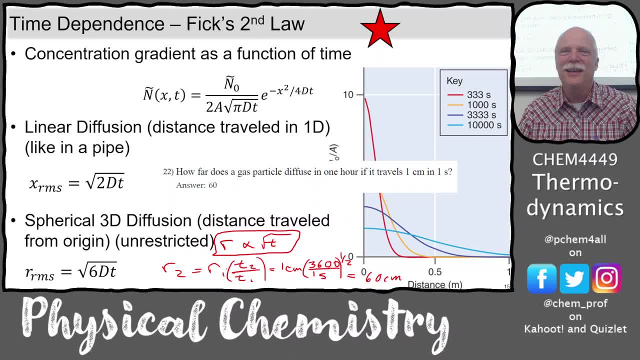 between the time I've done it before and I always come into class cold so that I can work my way through it slowly, you know, and it makes me think every year that's the best problem ever, because it's such a weird combination of electrochemistry and ksp and equilibrium and everything like that. 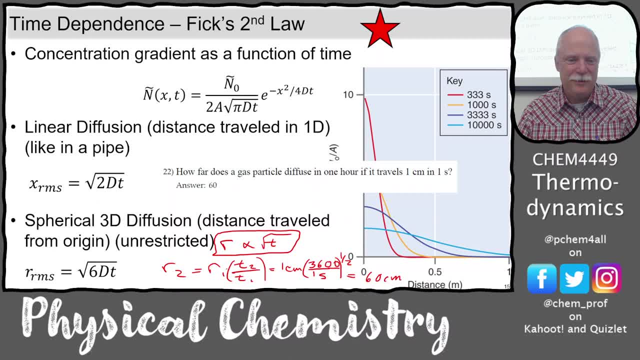 so it's a little bit, I'm just cleaning things up for these problems, okay, okay, all right. so let's do seven, six first, you said six, yeah, and let's make sure that. yes, there you go. yeah, it worked okay. okay, that's not, that's strange. 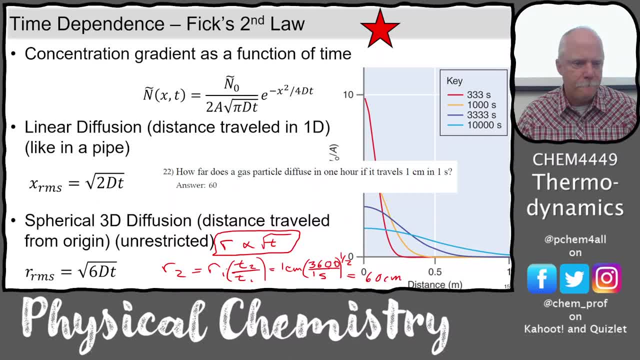 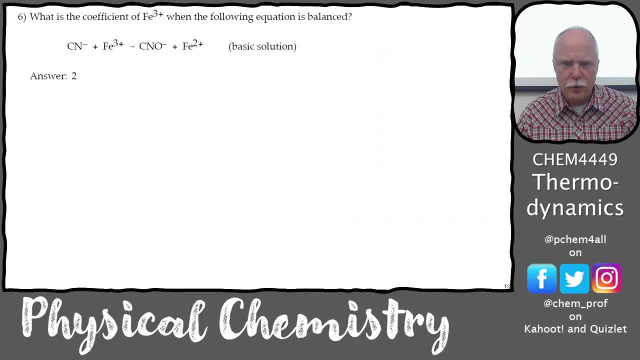 okay, I'm just making sure the video records what I do on the screen. okay, I think we're ready to go. okay, so this one, we're going to just want to break it into half reactions that the iron one should be really straightforward. so I'm going to sit up here and I'm going to do this one, and I'm going to do this one. 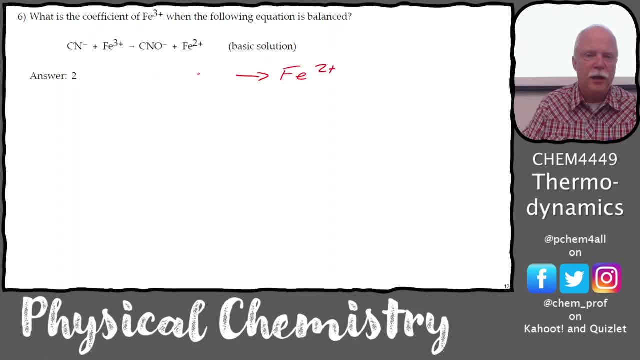 because I'm going to Fran's one as well, so I'm going to do it one more time. okay, this is called the long Bunge. this is a n wine is equal to two. so we're good. so that one's balanced, okay. so then we on. 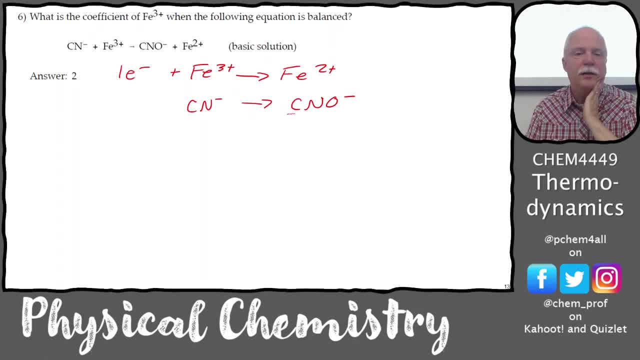 this one. we have the same number of carbons, the same number of nitrogens, so we have to just jump right to the waters, adding waters to balance the oxygens. so we put one water on this side, so the oxygens are balanced and that is added. 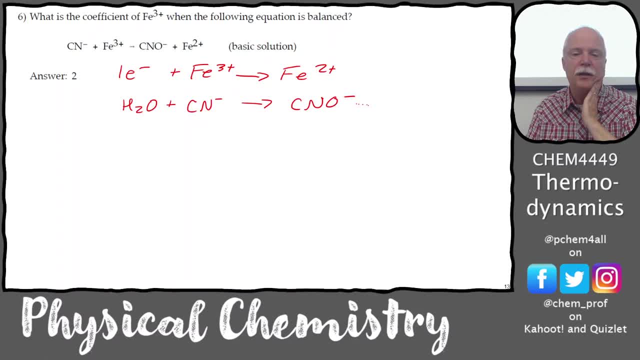 hydrogen, so we need to add in some H plus, so we have two of those we need to add to H pluses. so now the hydrogens are balanced and that changed the charge. and so now we need to add our electrons, minus one on the left, plus one on the. 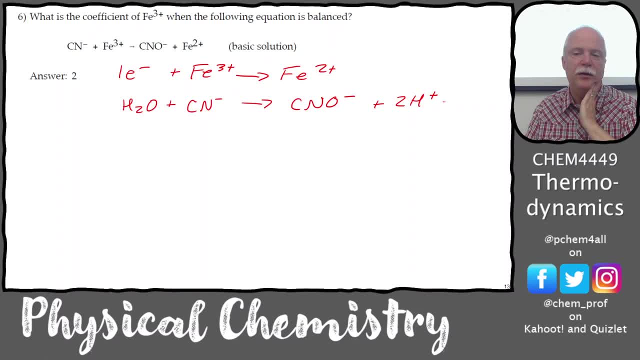 right, actually, because they've got two minus one. so we need an electron here, okay, so does that work? or do we need to be two electrons, don't we? okay, so I'm gonna have to multiply this top half reaction by two, and then they'll bring it down. so this is in in basic solutions. 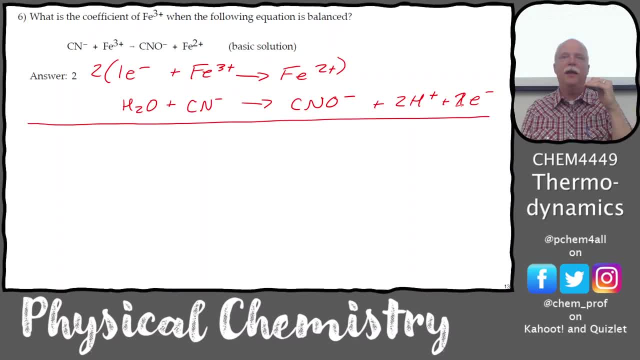 so we're gonna balance it just like normal and then we're gonna make it basic. so that's how I do it. you could, instead of adding waters, if you're gonna do it in basic solution, add hydroxides, but So this is a more consistent way to do it. 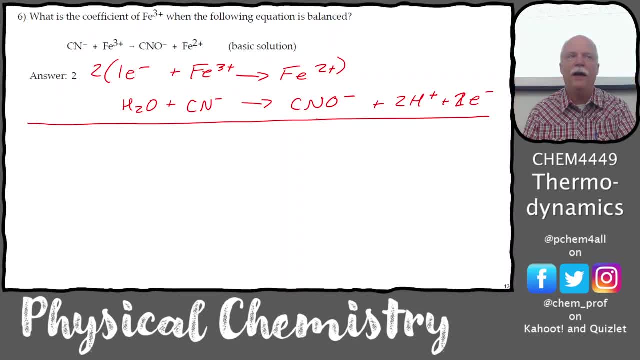 It may be longer, I don't know, but I do it this way so I don't ever have to change how I balance an equation, And then at the end I do, kind of like mentally, I do an acid-base titration. 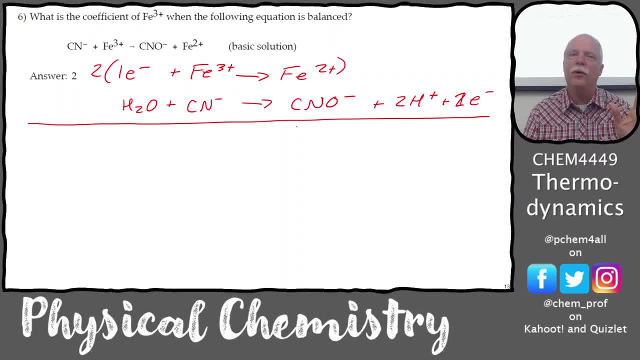 I add as many bases to both sides as I have photons, So let's go ahead and bring everything down. The electrons have canceled. We have two electrons on each, so we don't bring those down. But we have two, three plus plus H2O, plus Cn minus. 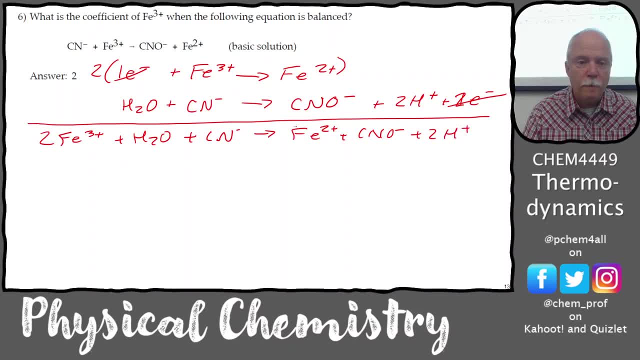 Okay, so this is what I missed, Thank you very good. Yeah, that's where you mess things up. And so then we're looking at this and we say, okay, I've got acid protons as products and I want to pull this reaction forward. 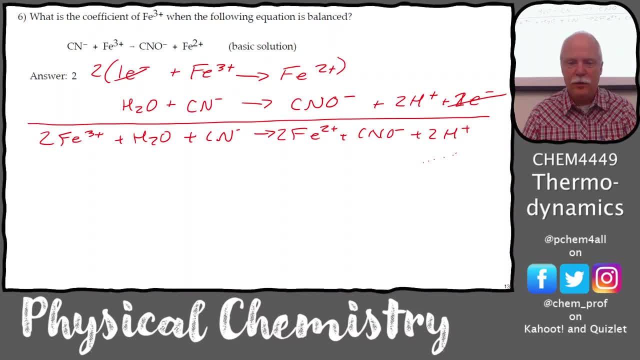 And so if I put it in base, that's going to pull it forward. So I'm going to add in two OHs right here, to both sides, Okay, so they come along here, And so these produce two waters, Right. so acid-base neutralization, and then my hydroxides show up as reactants. 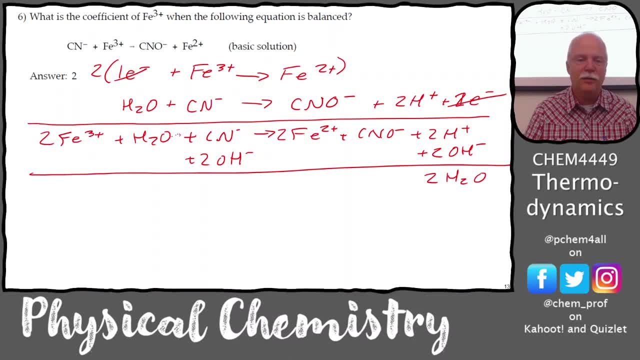 But I've got water on both sides and so I want to cancel those. So I want to cancel this one water with one of these waters, And then everything else works out. So two Fe3 plus plus two OH minus plus Cn minus plus two Fe2 plus. 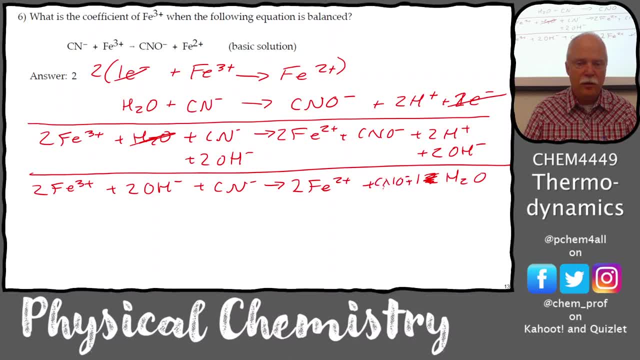 So that's pretty straightforward. That's how I do. basic solution redox reactions is I just balance them normally and then neutralize the protons and cancel the water. So it's really two more steps, But it's a nice, conceptually easy step. 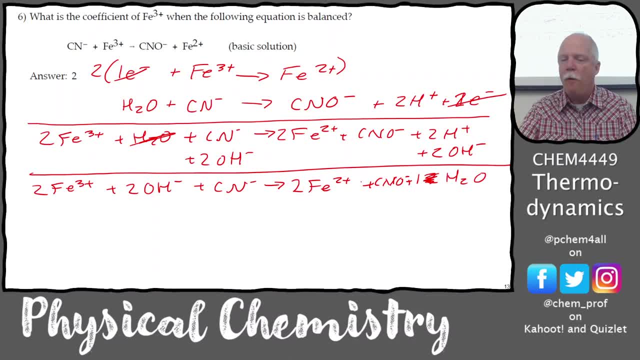 So, And most of the redox Redox reactions that I've come across have protons as reactants, So they take place in acidic solution. But if you have one that takes place like, if you have one like this where the acid protons 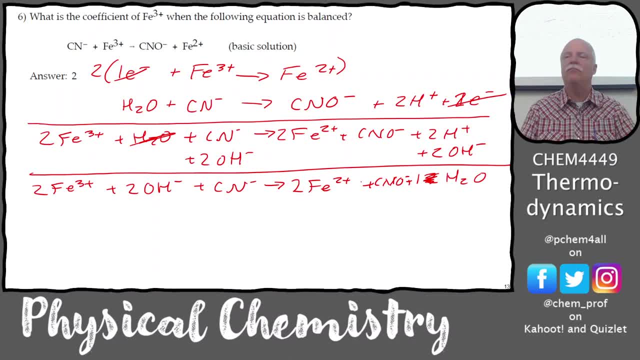 at the end of the balancing show up as products. that's going to be pushed forward in basic solution. So that's how you know if a redox reaction is a basic one or an acidic one is what is? what's in the reactants, what's in the products? 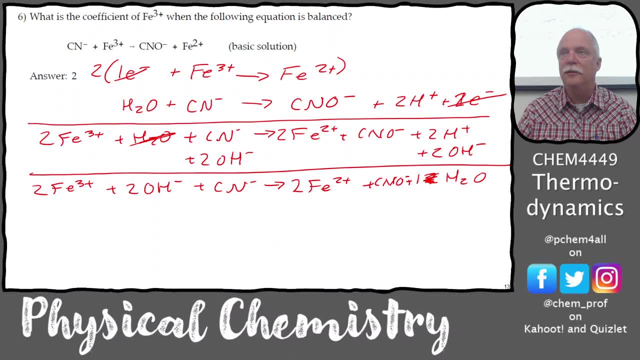 Some of them are really mitigated by very shortly. Okay, Okay, Okay, Okay, I'll give you a sample of fire. This is the first one. Okay, We have a lot of fire here. Okay, Let's see. So these are the two redox reactions that I have. 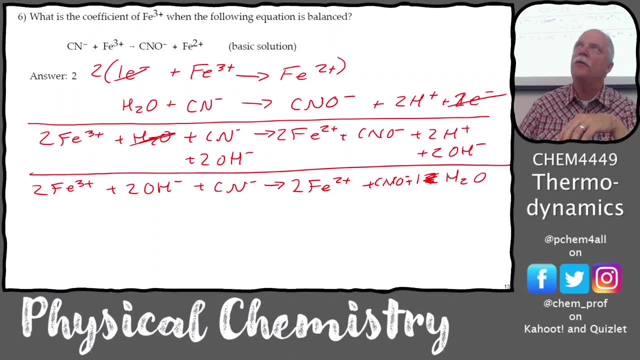 They're alreadyじ Okay, Are very strong acids, So there are like bacteria extremophiles. I guess that will get in and they will, Let's see. I guess that's a produce acid water and so that's what acid mine water is. it comes from bacteria. so what keeps it from? 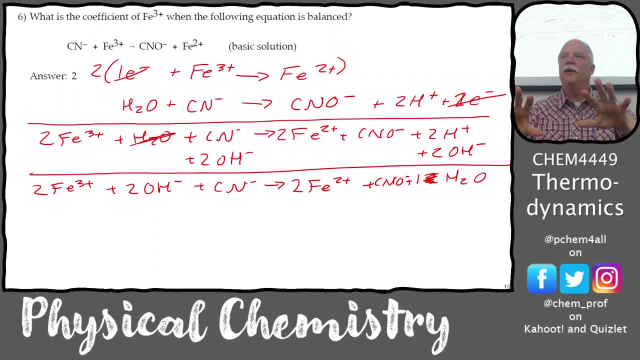 happening naturally. well, you've got to have oxygen in there, and so it's when we do mining we open up all of those deposits of iron pyrite to oxygen and the bacteria love it, so they start growing on that iron pyrite. so a lot of places in colorado are super contaminated because of. 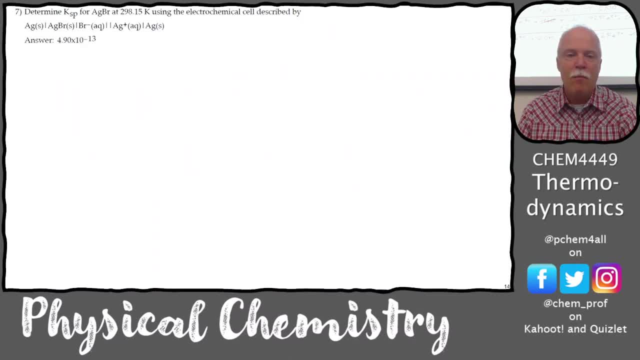 this and it's just natural bacteria and oxygen. okay, let's do this crazy one, okay? so this is talking about a case ksp for agbr using the electrochemical cell. so this has everything in it. it's got the line notation, all kinds of stuff. so we've got to figure out what's. 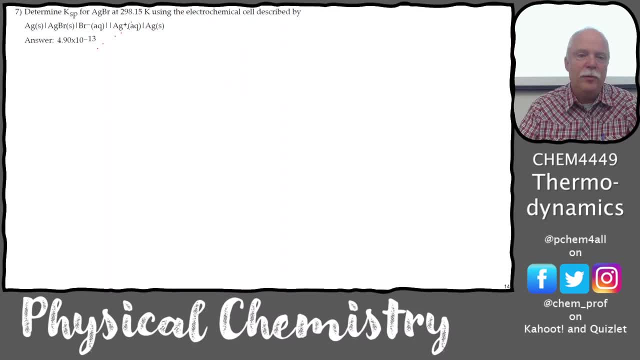 going on at the anode and the cathode. remember, this is in alphabetical order. so the very first thing is the anode. okay, and the anode takes place at the oxidation, or oxidation takes place at the anode, and then we have the reduction reaction and then we have the cathode. 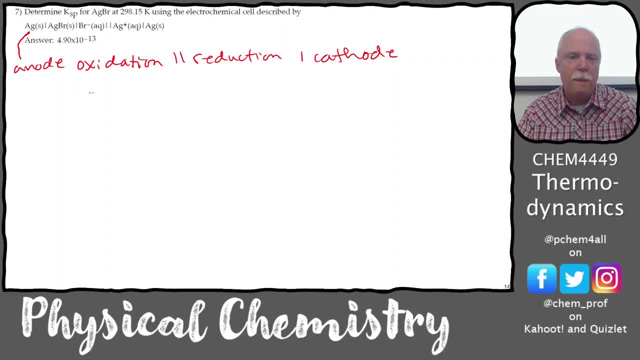 so let's write out, write out our half reactions. so notice this salt bridge right here. this kind of breaks the two pieces. so this, these three things here listed what's our half reaction. that's our first question. this one's easy, right, you gotta. you've got a half reaction. that's silver plus and silver solid. okay, so let's. 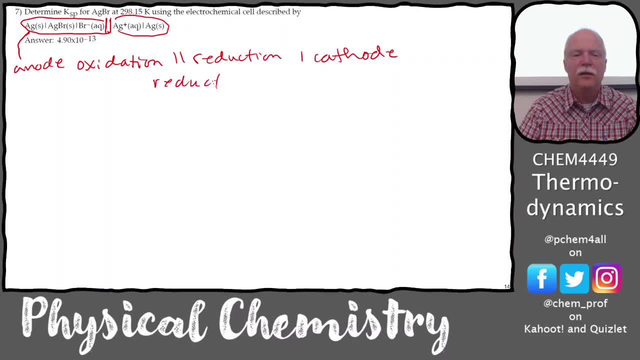 go ahead and write. let's write that out. first: reduction. so we have um ag plus plus. an electron gives a g solid. it's a reduction, it's gaining electrons. also the oxidation number is being reduced. it's going from plus one to zero. so that's the reduction reaction. so that's taking place at the cathode. now the 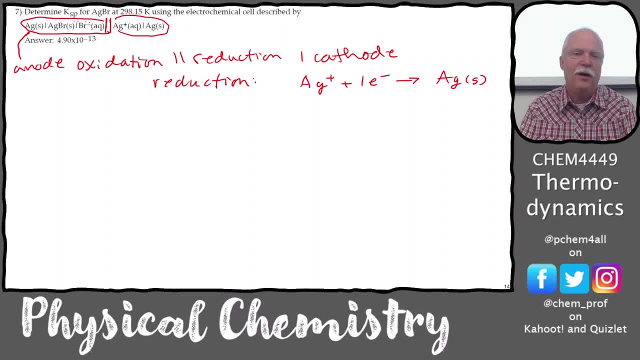 real trick is this one over here. so we've got to figure out what the reactants are and so focus on the bromine. so we have bromine attached to silver and then we have bromine ion and it's going to be an oxidation. okay, so we got to write that in in a way as, as it as, it is an oxidation, so let's just like over here. 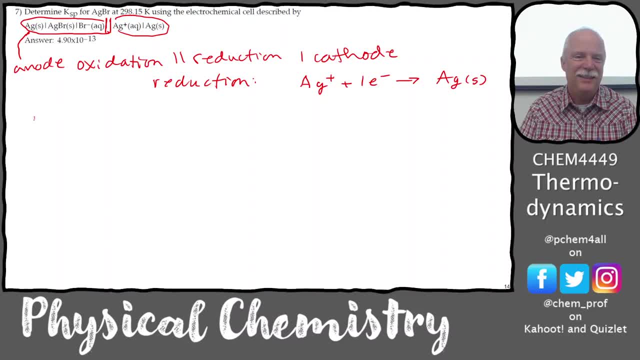 on the side do some scratch paperwork, okay, so let's balance this. we have ag br going to br minus aqueous and let's balance the silver. so this is agbr solid, this is br minus aqueous, and we need to balance the the silver, and notice it's in contact with that. 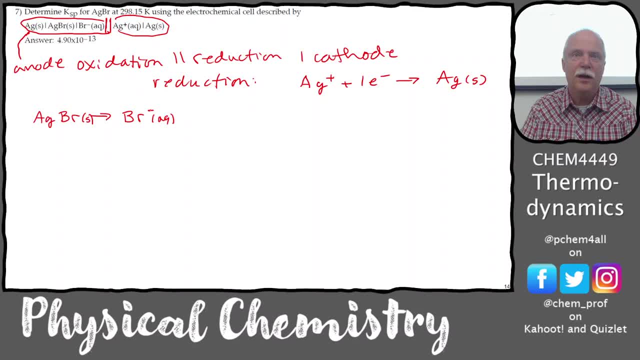 silver electrode, so it's probably going to be silver solid, okay, and so we're looking at this reaction and we're trying to figure out. well, how do i write this as uh, how do i, how do i write this as an oxidation? so we, we don't have any oxygens. 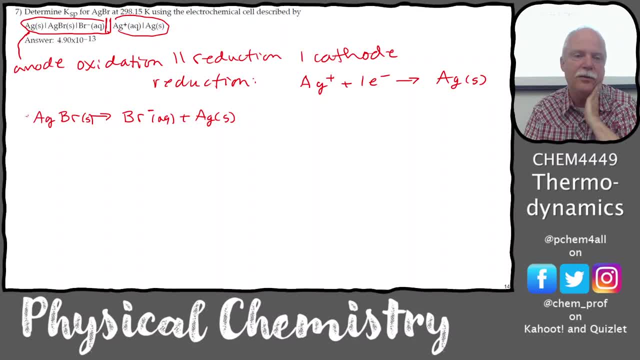 we don't have any hydrogen, so we're left with the electron. so we got to put an electron on the left, right, left, not right, left, correct, okay? so if i were to write this over here on the right, as it is, it will be backwards. we need an oxidation, and so i've got to flip this whole thing because we 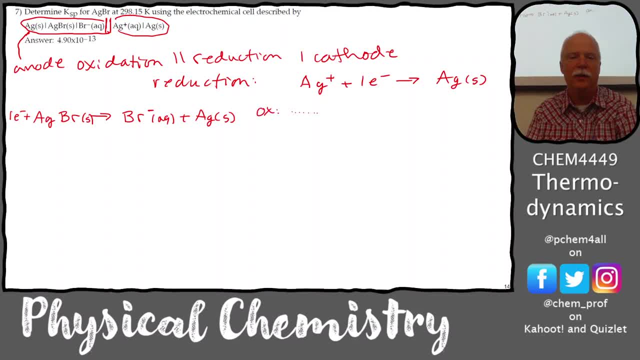 need a reduction and we need an oxidation reaction. so i've got to reverse this thing and write it with the agbr solid here plus one electron, and then we have br- aqueous ag solid. did i get everything? yeah, i got everything. all right. so that's our electrochemical cell, the two half reactions. 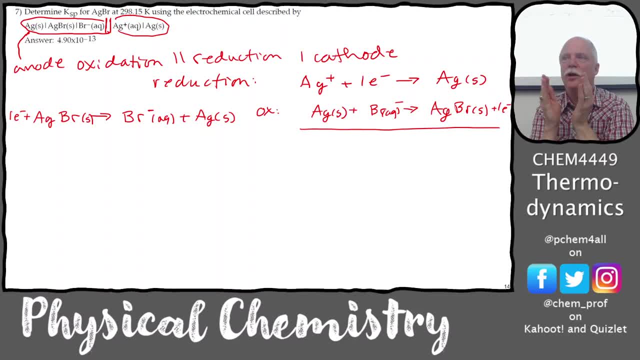 what would have? what stops you like up to this point? have you did? were you able to get this far? i guess yeah. so if you go digging around in the reaction table, you might find these two reactions and you compare them up, but i was just trying to go from the line notation in case we didn't have that table. 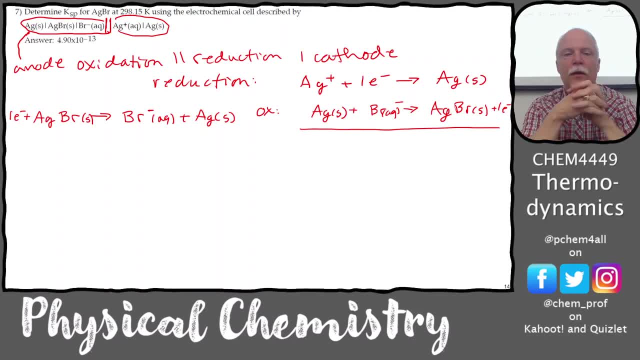 now we're going to need the table for the numbers for sure, yeah, but anyway, that did that make sense, though. we need a reduction and we need an oxidation, so we have to have the electrons on opposite sides of each other, and so then i have. that's why i. 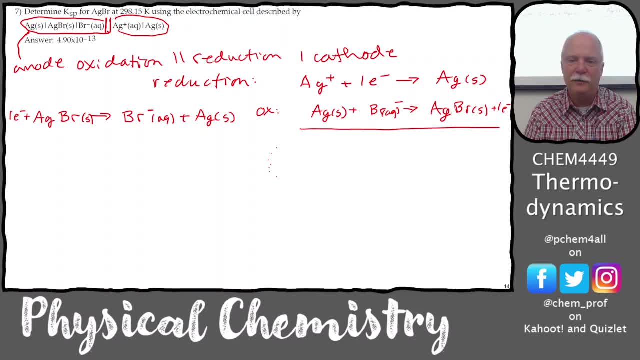 had to flip that reaction. so then we we go ahead and cancel everything down, and this is the cool thing. so the electrons cancel, that's fine, but look, the silver solids cancel, and that's pretty cool. we're left with Ag plus aqueous, plus Br, minus aqueous, giving Ag Br. so which is? 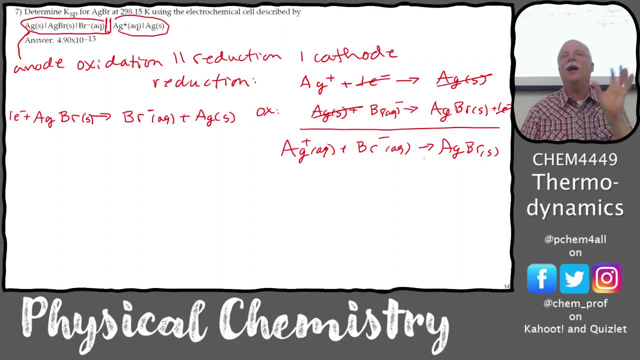 our KSP type. you know, solubility problem backwards. okay. so if we can get the equilibrium constant for this, if we reverse this reaction, it's one over that equilibrium constant. so this is going to be a spontaneous reaction because these two things precipitate out. so it's going to be an equilibrium constant, that's. 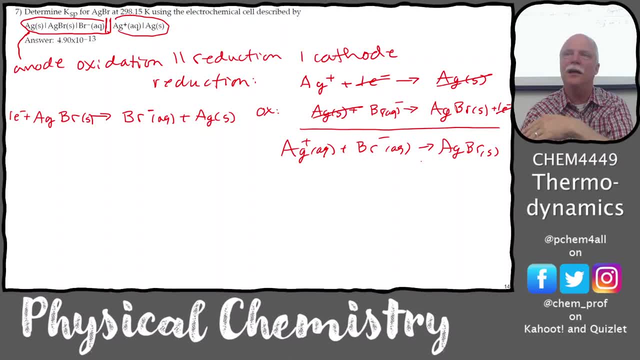 that's large because it's the lies to the product side. but if we flip that, the equilibrium constant is going to be really small. we'll have the KSP for silver bromide, and so all we have to do is measure the voltage of this cell. we 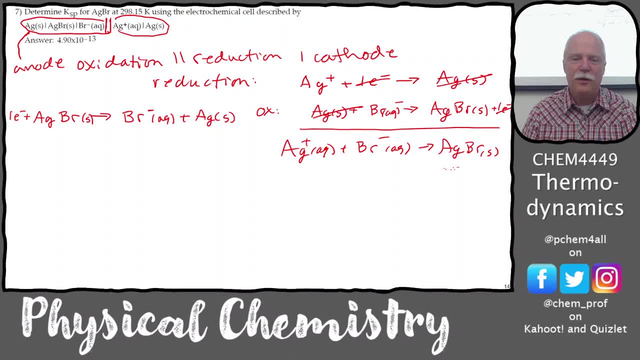 get the KSP. that's pretty cool, so let's go ahead and do the the voltages. so let me just make some space here for it. so what is the the voltage for this first reaction from the table? you Yeah, um, do I need to pull up the table that you'll have on the exam? 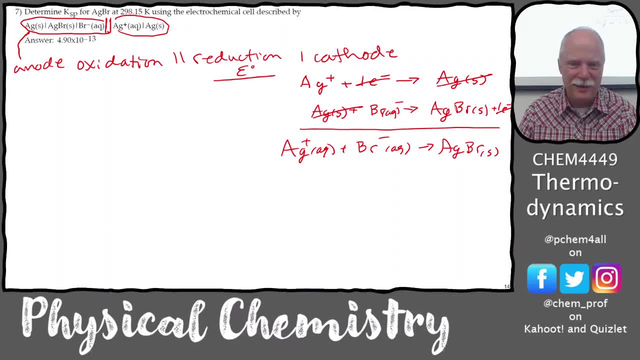 okay, let's see if I get it's probably. I think it's on there, I'm not sure. let's see it's 0.8 for the silver iron. um, okay, So let's go ahead and do that: 0.8, plus 0.8, that's a reduction reaction, so you don't have. 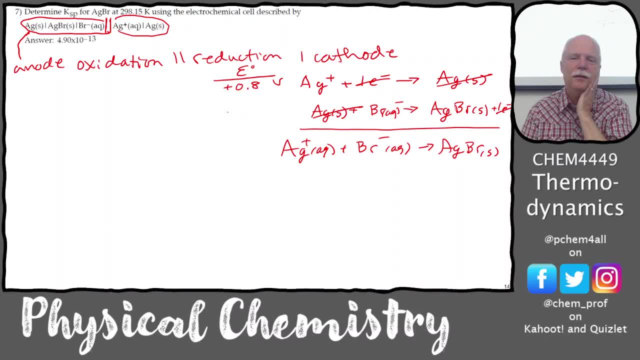 to change the sign. For the next one we'll have to change the sign. I'll try to pull up that table. I've got so many files on my computer. it's crazy. thermal and redox tables. there we go. Okay, where are you? 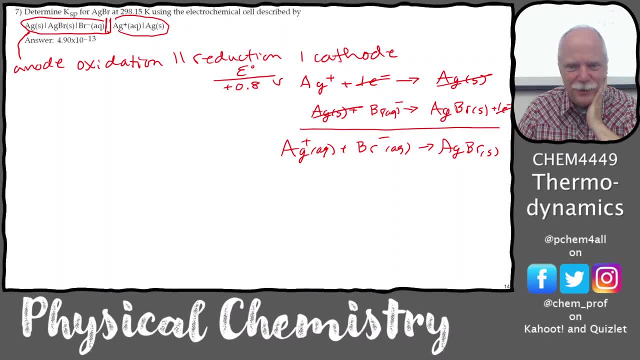 Yeah, it's not on the exam one, because I don't ask this question on the exam, so I thought it might be It's not in the class one either. Let me pull up the textbook. yeah, I've got a PDF of the textbooks. 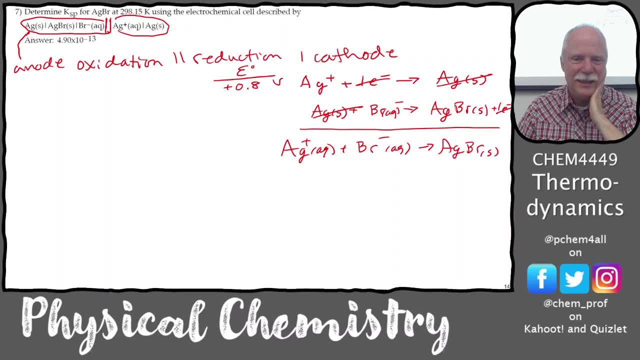 Thank you for being patient. Here we go: reduction, half reactions. they're not sorted, of course. I mean they're sorted in terms of decreasing. okay, here they are. they're sorted in alphabetical order, found it, So let me grab a snip of that, just so you see what I'm looking at. 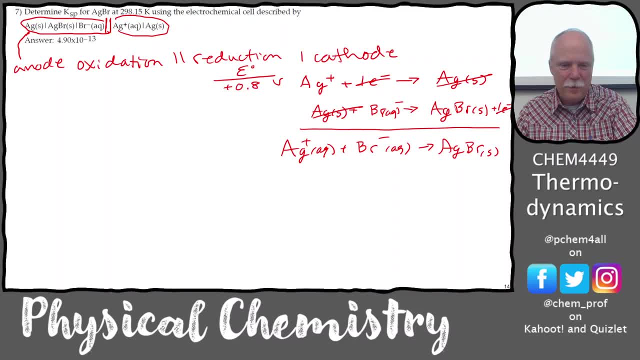 Okay, Let's see which one is that That's on the discuss, Did it appear? Yeah, Okay, good, All right, here we are, so let's go back to the slideshow, All right? so we're looking at this table and we can see that it's 0.08, but it's written. 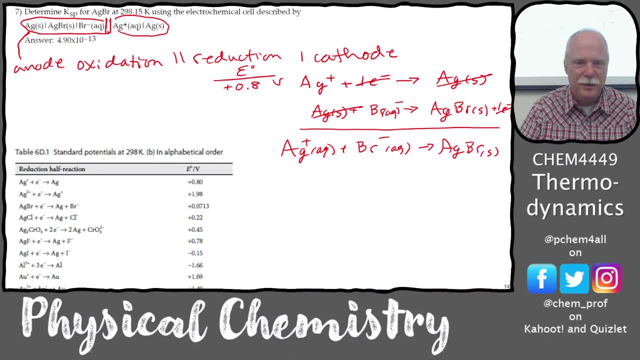 in reverse, because it's an oxidation reaction. So it's minus. Let's see It's 0.0713,. I don't know, I don't need all those extra decimal places, but volts And so so that would be 73 volts. 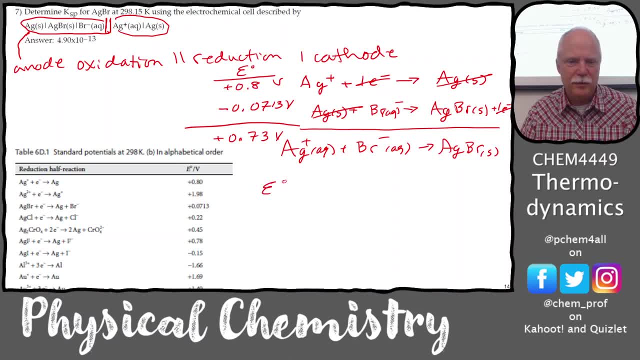 All right, So that's the E7.. Now, if I take and place a cell, How do I get to equilibrium constant? Because we want the equilibrium constant. This is a great problem. We've got to figure out what the oxidation and reduction reactions are. 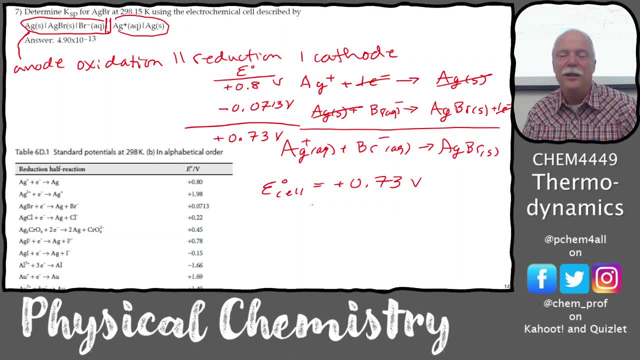 We've got to use line notation, We've got to find the cell potential, But we still aren't to the equilibrium constant, The, what, The supplement, The, what The cell potential, The, what, The represent. think about where we so, let's, let's work backwards. we want to get the. 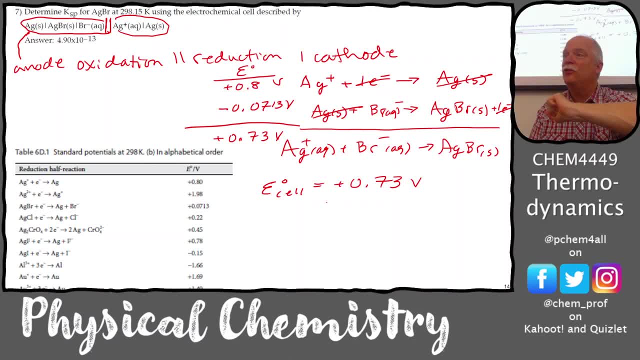 equilibrium constant. what value can i use to calculate the equilibrium constant? um well, think about this. we've got the reaction written out here and so, um, okay, let's do that. so we could say k is equal to the way it's written. one over the concentration of silver ions. 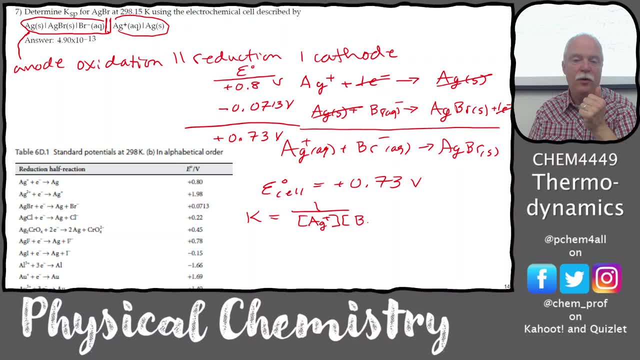 and one over the concentration of bromine ions. so that's k, right, that makes sense. that says we've got the reaction. that's k. um. you know, one over that would be ksp. that's ksp, that's ksp. that's where we're actually getting to in terms of the problem, right? so one over that, so. 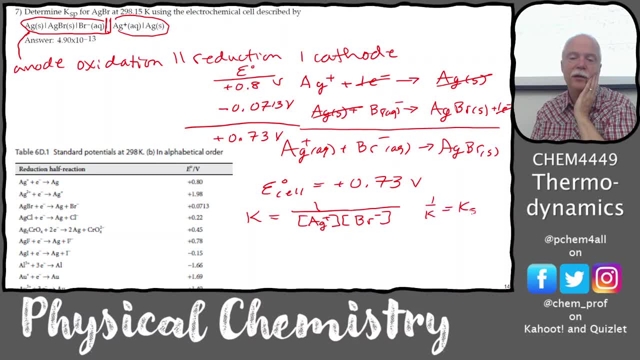 one over k would equal ksp. so that's the end of the problem. when we get there, how is e cell related to k? that's the. that's the trick. is e cell related to any other thermodynamic values that we could use to get to k? 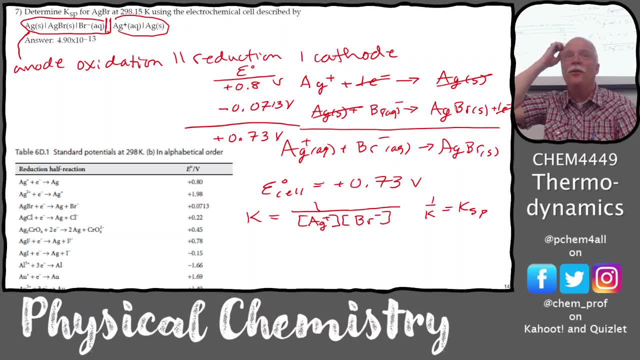 delta g. that's the one. so we've got to go through delta g to get to k and i've got e cell. now i can calculate delta g, okay, so let's go ahead and write this out: delta g. i'm just write it up here in the corner. so 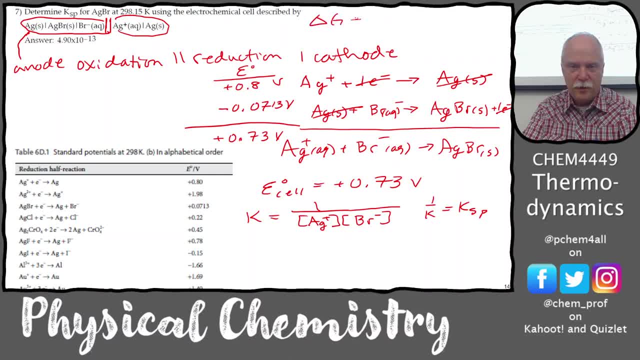 delta g is equal to um minus rt, lin, k. so that's the delta g relationship to k. and delta g is also equal to the e cell equation. what is that? one minus nfe? so there's my, there's, there's my connection to k. so from this positive 0.373 i could calculate k, sp and ksp. 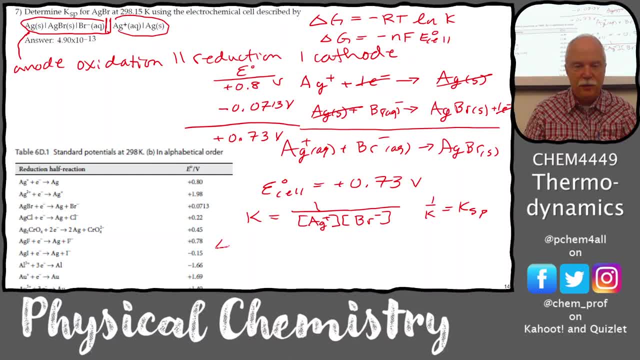 so i could calculate my, my delta g. so delta g is equal to minus. what is n in this case? so i'm looking at this reaction. since i've balanced this reaction, i know what n is. it's the number of electrons exchanged. so that's one, Okay. One mole of electrons. Faraday's constant is 96,485 joules per mole, per volt. Okay, And then I've got volts here plus 0.73 volts. 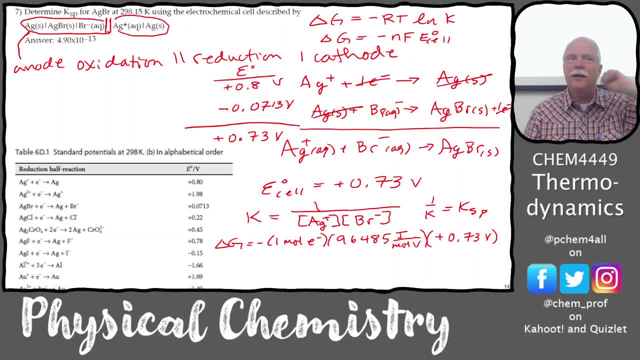 So my volts cancel, my moles cancel and I've got joules for my Gibbs free energy And it's negative because I have a negative sign out front. So I've got a nice spontaneous reaction. So I could have asked you that question too: What's the Gibbs energy for this reaction? 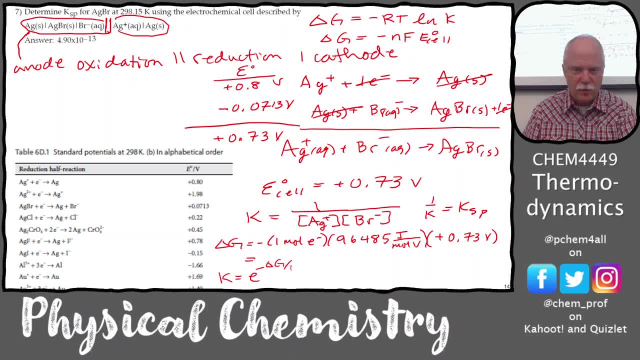 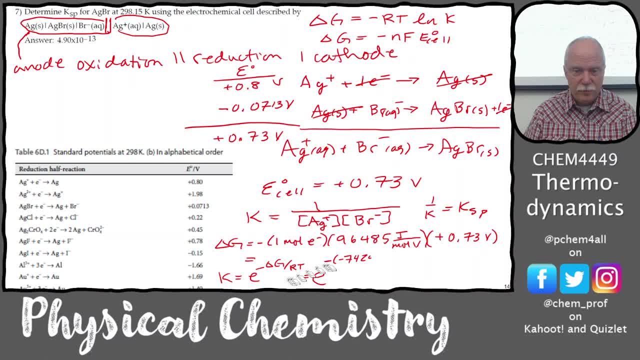 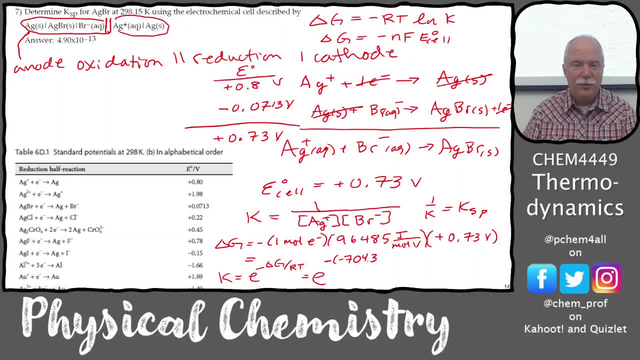 Hey, hello everyone. I'm John from Strangler's- unusually great and full of who to get it to the kids. Do you want to network me? Yeah, I have got a computer. Thank you, not just to the ones place, it's fine. we started with two significant figures. 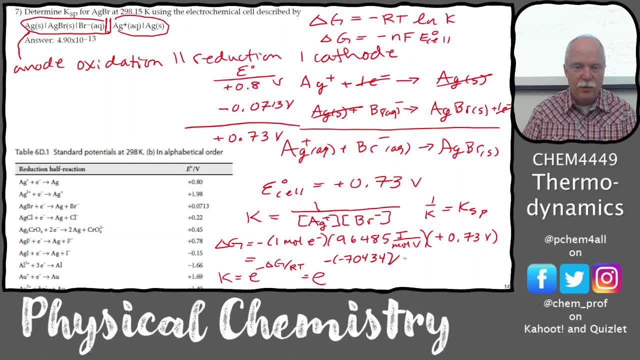 all right, so that's that divided by 8.314. so that's joules. let's go and use our unit so we don't screw up. that's in joules, correct? yeah, now there's always this discomfort here. that's joules because we calculated, but you know it's for one mole of all those substances. so 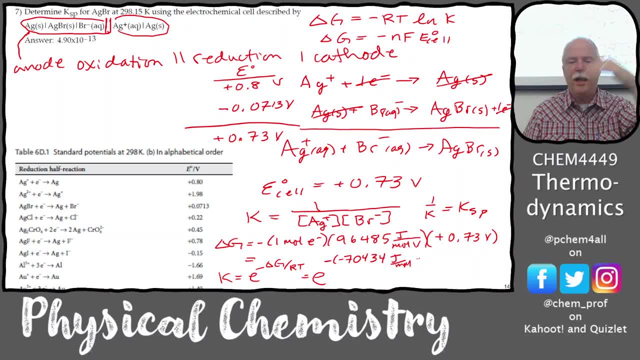 there is an implied per mole here, so that it'll cancel the per mole and the arc and the gas constant. so don't be um. that always gives me heartburn too. it's like i have joules and now i need to cancel the mole. right, but it is for one mole of the ag one. 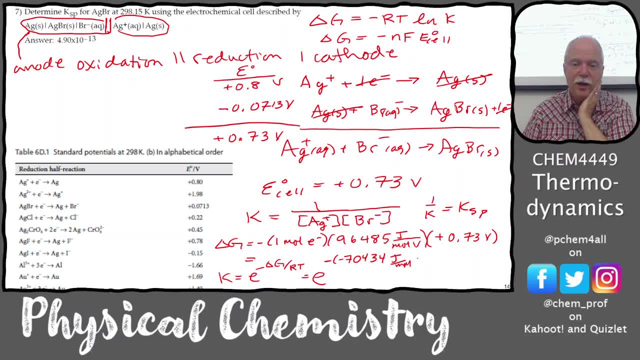 mole of the bromine, one more than agbr. so there's an implied per mole there, so divided by 8.314 joules per mole kelvin. and then that denominator has a 298 energy temperature, so it's divided by both those numbers multiplied by each other. 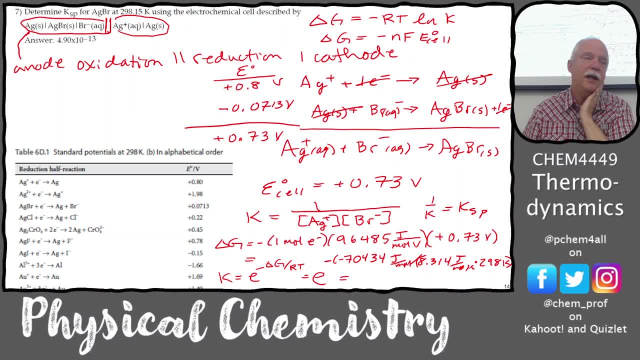 okay, so that's a long calculation, but notice the negative signs: cancel. that's the really important piece. what'd you get? 2.2 times 10 to the 12th should be big because it is a insoluble substance. so. so it's going to lie to the right right, so that's good. 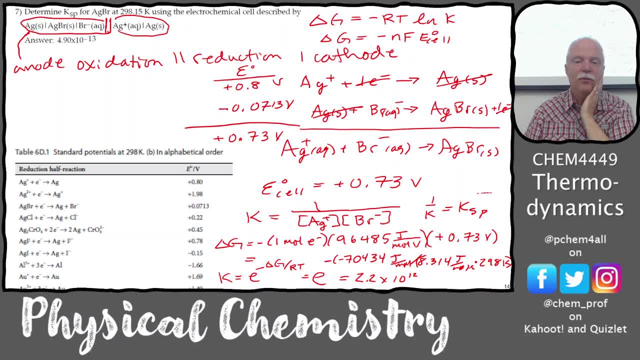 and so then we take one over that. see this, this equation here: one over that number is the ksp. so we got the right answer, so we got the right answer. so we got the right answer, so we did it right. so it's close to two. so one half would be point five. 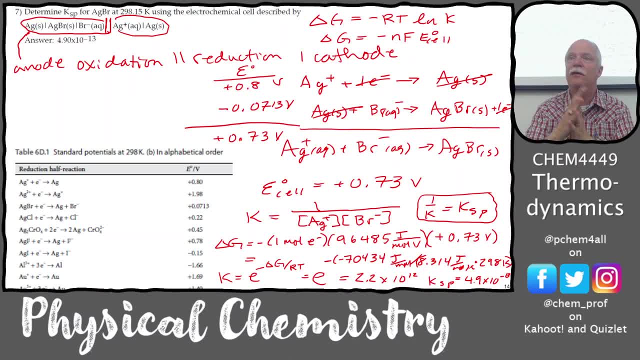 and so that's where we get the 10 to the negative 13. we had a 10 to the 12. so it was like 0.5 times 10 to the negative 12. and so that's 10 to the negative 13. so that's fantastic. 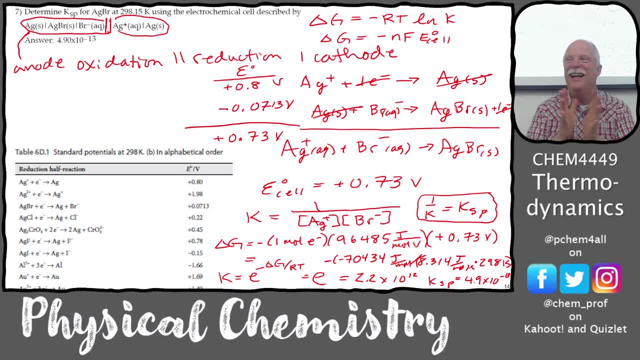 what a long problem, but that's why it's on the homework. am i going to give you this whole thing on the test? no, because you wouldn't finish the test. but isn't that a great problem? that is just beautiful and it's everything in it: gibbs, energy equilibrium, constant ksp- for goodness sakes, that's. 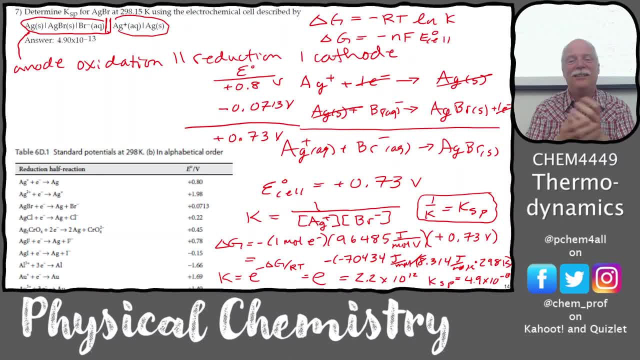 gen chem 2.. and that's also a really neat way. if you had this electrode set up with silver and bromine and everything that, you could measure the ksp electrically right, because i always wonder how do they measure these really small like 10 to the minus 13 uh ksps, you know, are you really going to? 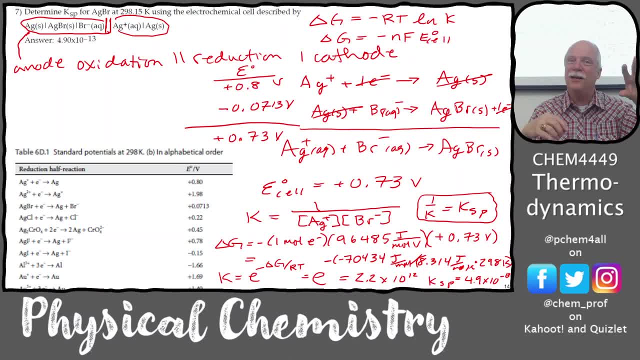 measure the concentration of bromine ion in that solution down to 10 to the minus 13.. that's a really small concentration. so how would you measure that? well, electrochemistry is a way to measure some of these things, so it's kind of a gee whiz type deal. it's like: okay, that's how you would measure. 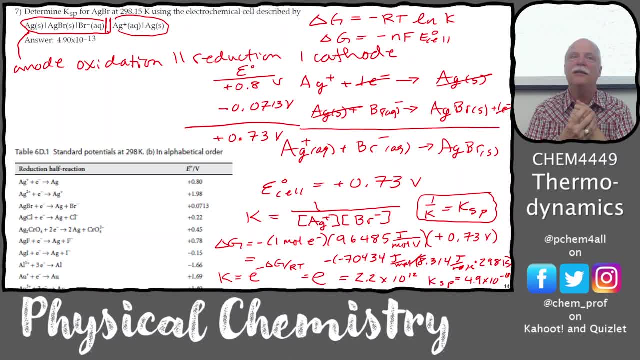 some of these really small reaction equilibrium constants. Cool, Which one? Okay, let me look at that. I can't find my mouse On number 12, 15?, Okay, Okay, so this is the thing We want. we get the biggest difference. 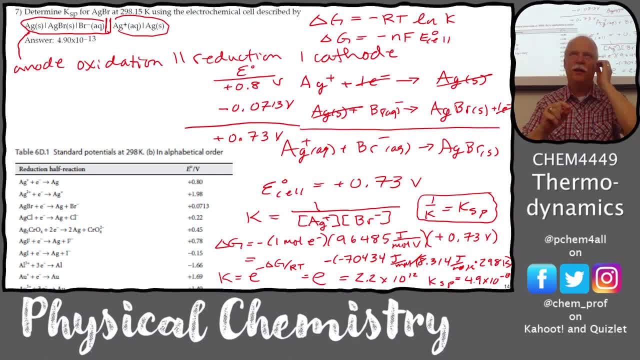 between. think about the differences. You want the largest difference in mass, but you want both of them to be as small as possible, So there's two things at play. So, yeah, you might have a big difference between two really heavy masses, but it'd be hard to separate them. 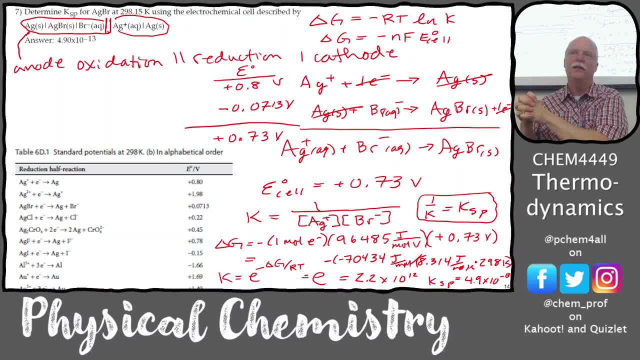 because percentage-wise it's not a big difference. So you want the largest percent difference. So going from like hydrogen to oxygen would be a huge difference versus well, is there another Like fluorine to chlorine Fluorine is, so that'd be 36 and 70.. 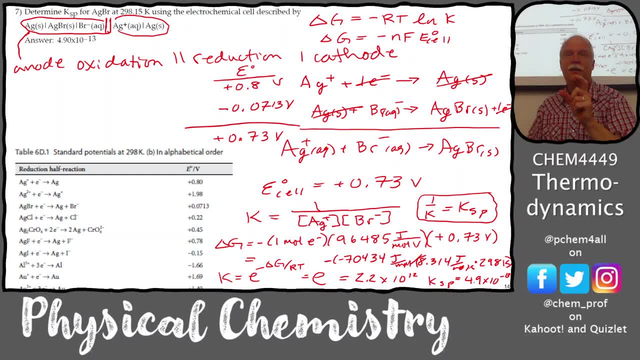 36 and 70 might be a bigger difference, but it's not a bigger percentage difference. Yeah, Okay, well, we're kind of out of time. Is there anything else that was just burning in your head? Okay, Are you comfortable with the ionic strength calculation? 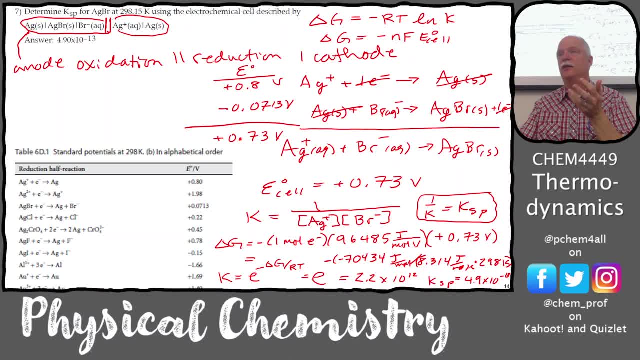 And and look at that, because I just wrote the test So I know this is on there. So look at the like the difference between the thermodynamic and the and the concentration rate constants. So let me just show you that real quick on this, this page. 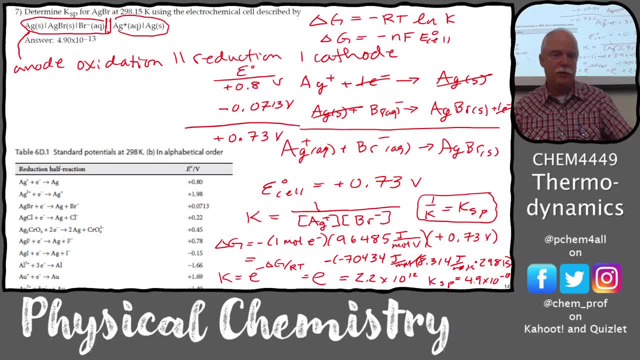 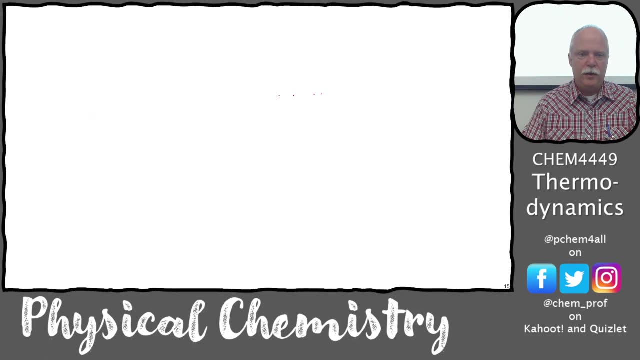 It's just kind of cool. So if I go to the next one, I don't know if I'll have enough stuff. next one, Okay, this will be worth it, So just stay two minutes later. Yeah, Okay. so let's just say for this generic reaction, 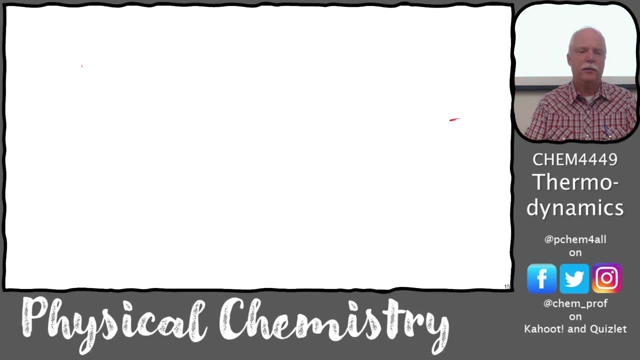 Okay. So you know if we have, let's try to do this quickly. A plus 2B is C, 3C plus 4D- crazy reaction, Okay. so K is obviously equal to the. it's the activity coefficient for C, cubed activity coefficient for D to the fourth power. 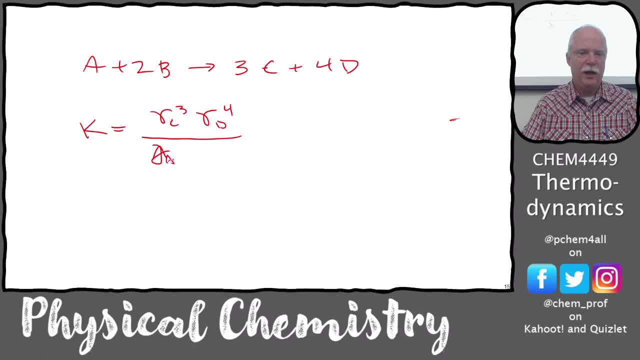 over the activity coefficient for A. So it looks the same as the concentrations, but the concentrations are over. are also there C, Q, D to the fourth? I might just wait to complicate it, but it's. it gets the point across really well. 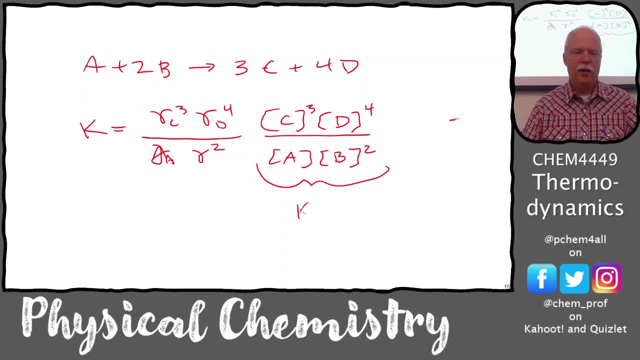 Okay, So this piece right here is K prime, The thermo. I mean, the concentrations are concentration. That makes sense. That's what you learned. And then this whole thing- because we've corrected that is the thermodynamic Thermal equilibrium constant. I just want to reinforce that, that.